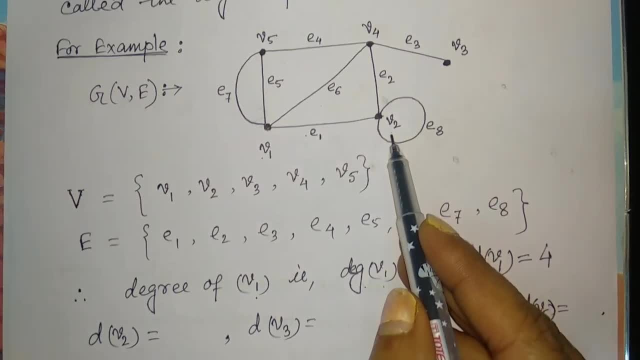 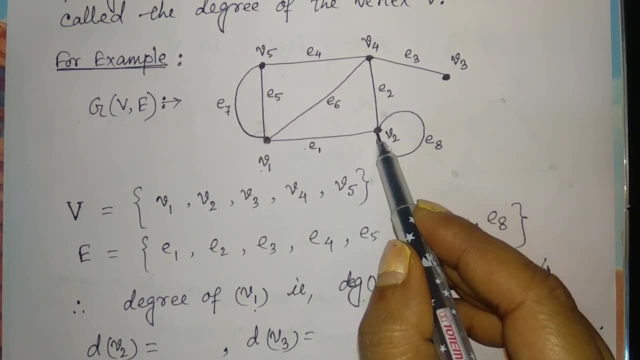 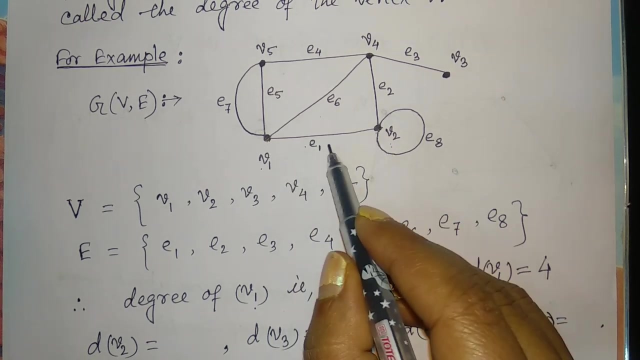 now come to the vertex v2. here. v2 here, look, one self loop is given. if any loop is given in a vertex, then for any loop it should contributes to the degree 2 to the vertex. actually, any edge means it have two endpoints. two endpoints means one edge contributes the degree 2 to the graph. 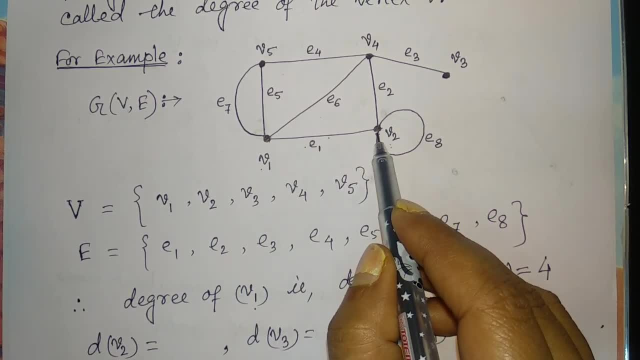 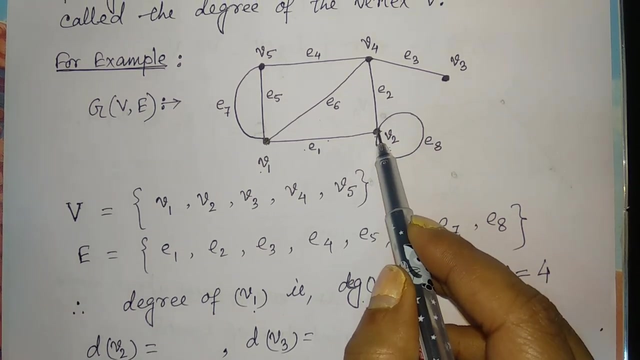 for both the endpoints one individual degree. if it is a loop, then for the loop starting and ending both vertices are same. for that reason we, if it have a self loop, then v2 get two degree for the self loop. so now if you want to count the 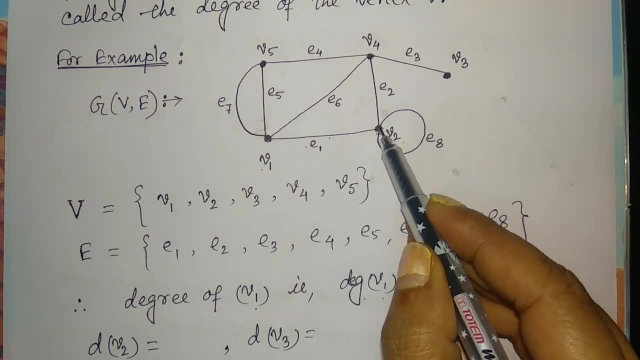 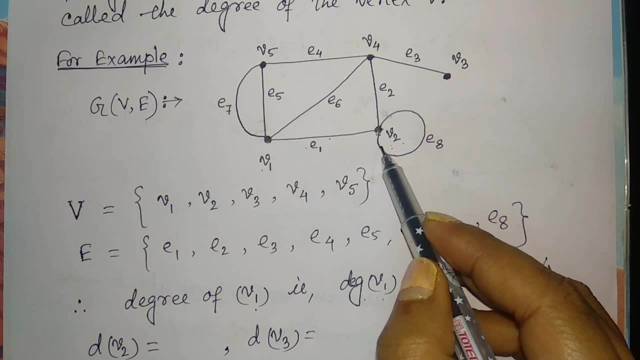 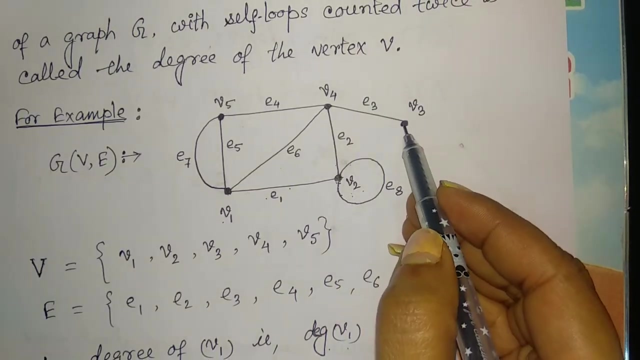 degree of the vertex v2, then its degree count is 1, 2 and for the self loop two more. so total 1, 2, 3, 4. so the degree for v2 is also. it is 4 now for the vertex v3. for the vertex v3 only one. 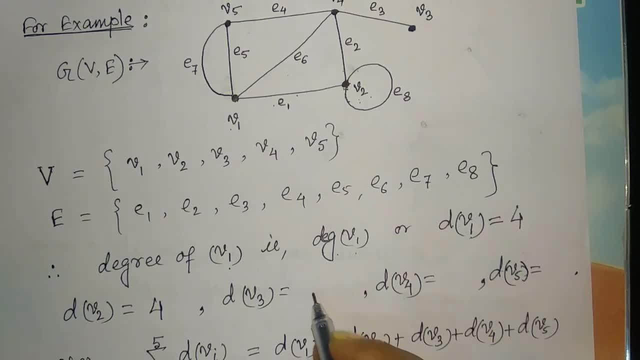 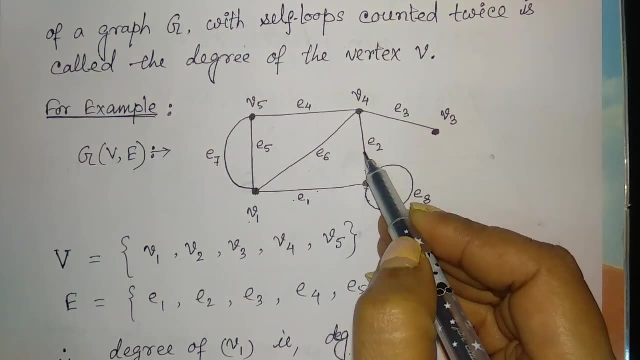 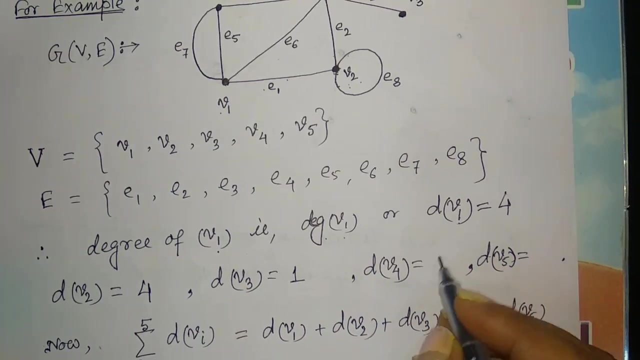 edge is in incidenting here, so that it is degree count is 1, only now the vertex v4. for the vertex v4 the total incidenting edges are 1, 2, 3 and 4. hence the degree for the vertex v4 is again for the vertex v5, 1, 2. 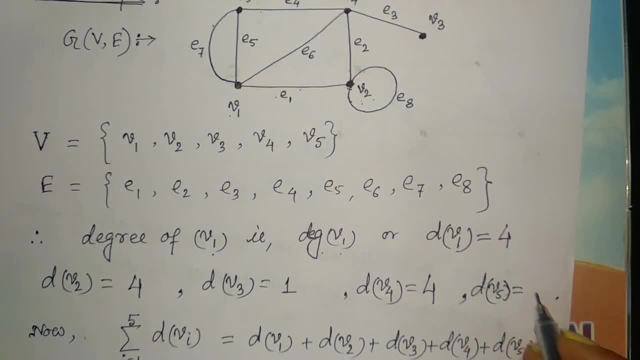 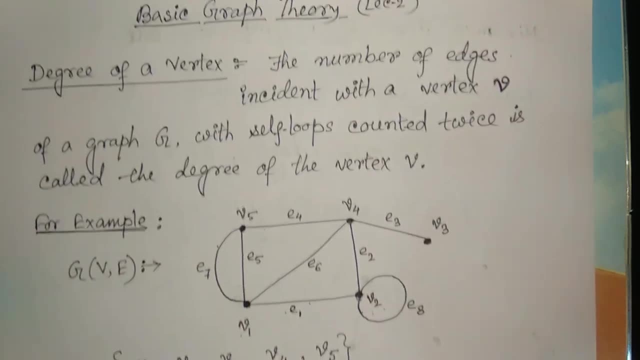 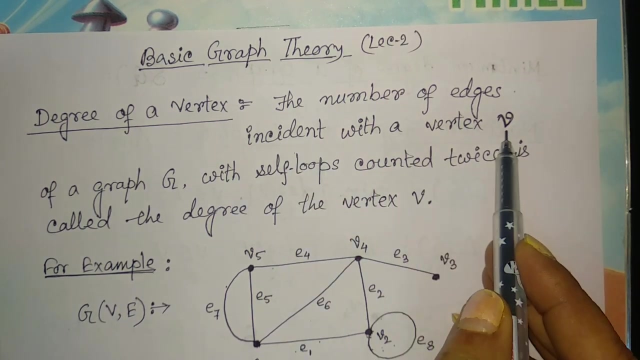 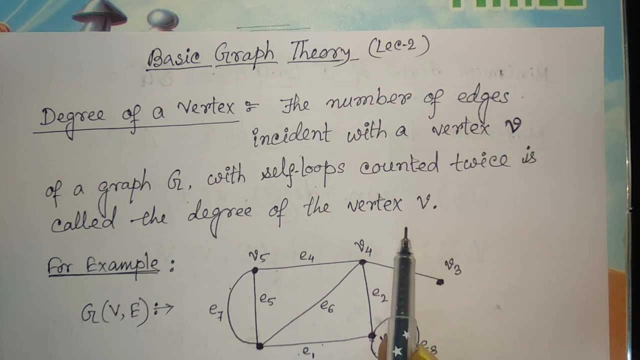 and 3. so the degree for the vertex v5 is 3. so this is the total Degrees for each and every vertex. For definition we can say: the number of edges incident with a vertex V of a graph G with self loops counted twice is called the degree of the vertex V. So now we 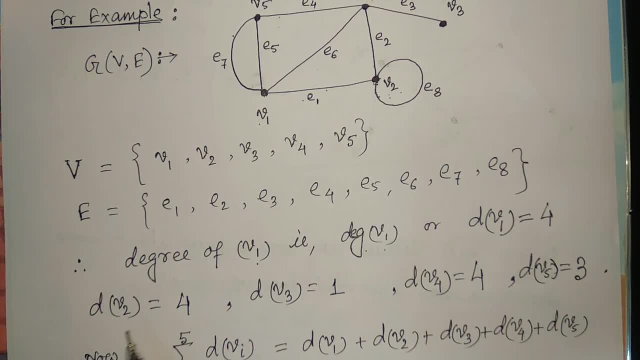 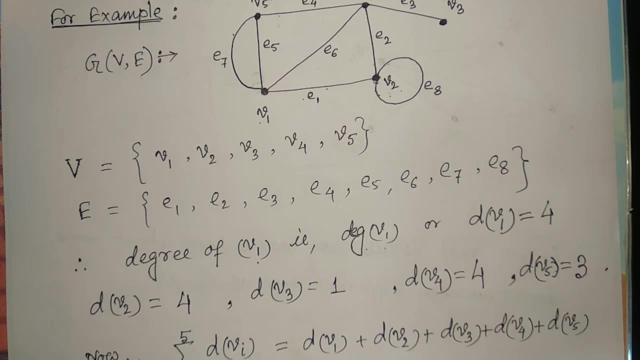 will find out that for V1 we have degree 4, V2 degree 4, V3 degree 1, V4 degree 4, V5 for the degree is 3.. So total degree count for this entire graph we can calculate by adding all those. 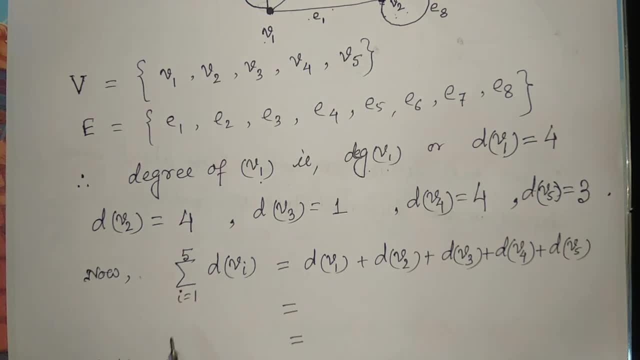 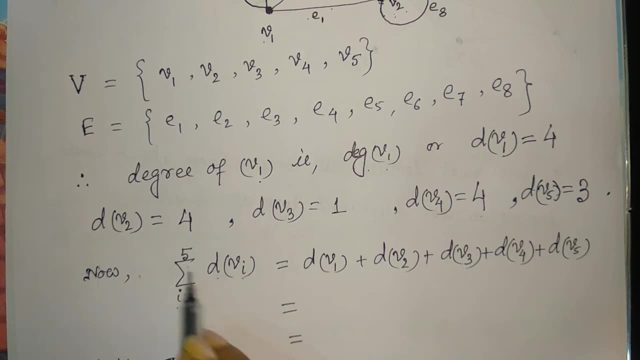 degrees. So the total degree count for the given graph is denoted by summation of degree of V I, where I from 1 to 5.. So it is degree of V1 plus degree of V2, plus degree of V3 plus degree of V4. 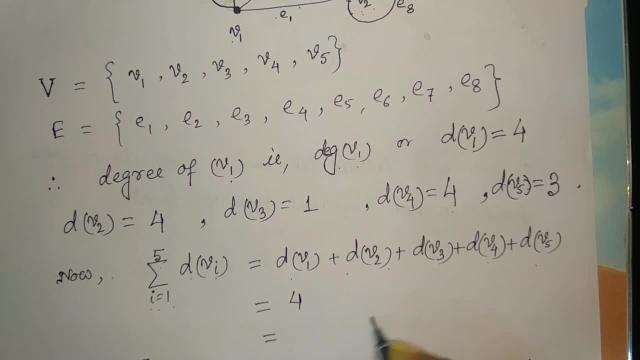 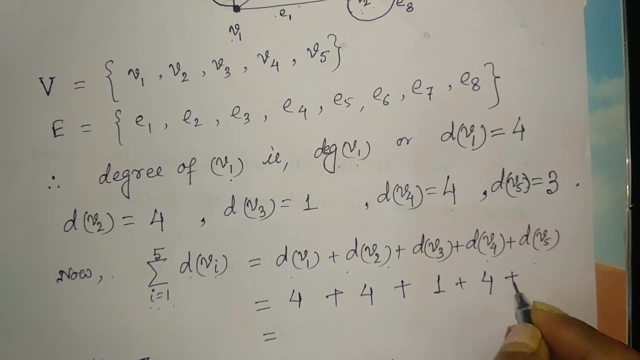 plus degree of V5.. So degree of V1 is 4, V2 is again 4, V3 is 1, V4 is 4 and V5 is 3.. So the total degree is 4 plus 4, 8 plus 1, 9 plus 4, 13 plus 3. 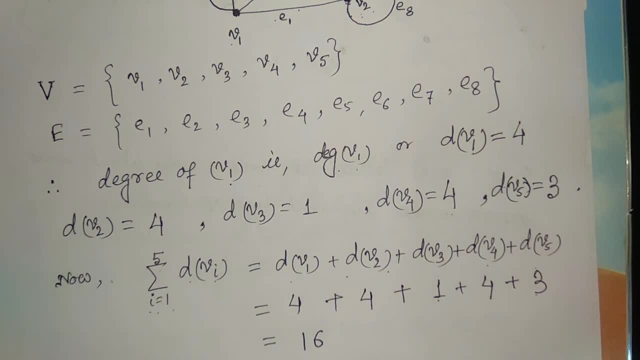 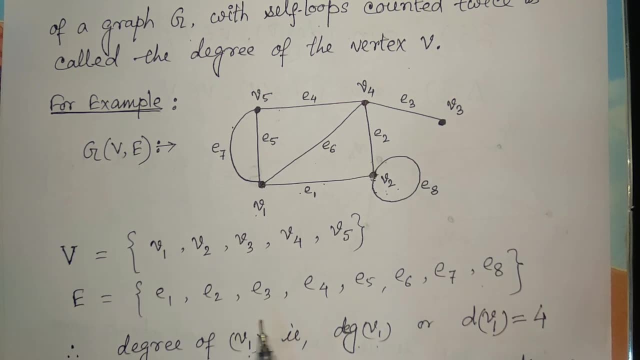 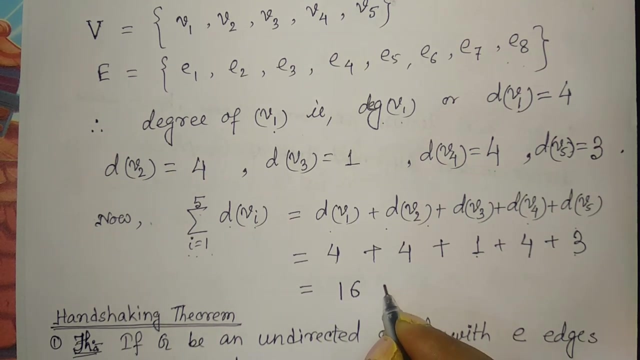 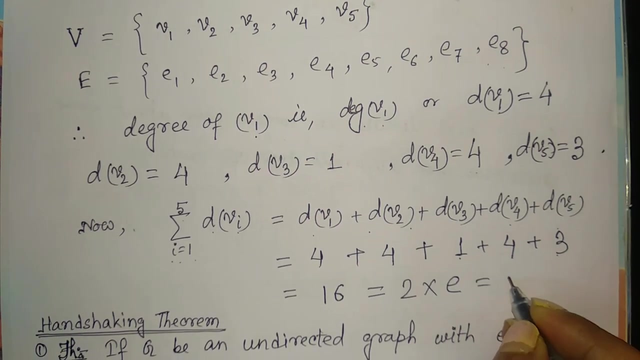 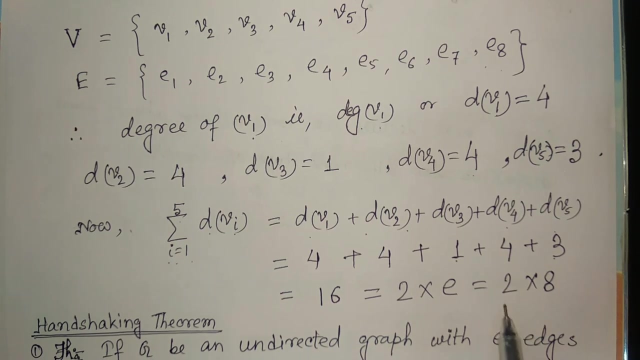 it is 16.. Now look how many edges are given in this figure. Here total 8 edges are there, So total 8 edges and the degree count is 16.. So that we can say 16 is actually the 2 into the number of edges That is here it is 8.. So total degree is just the. 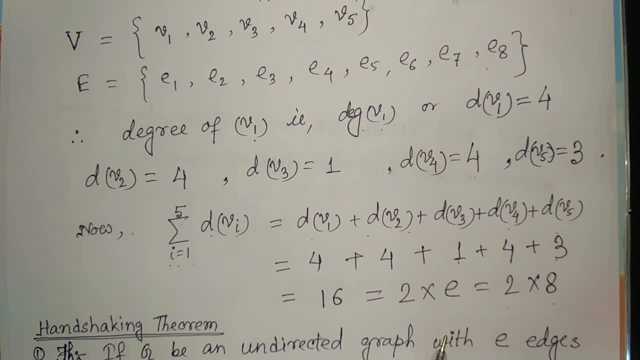 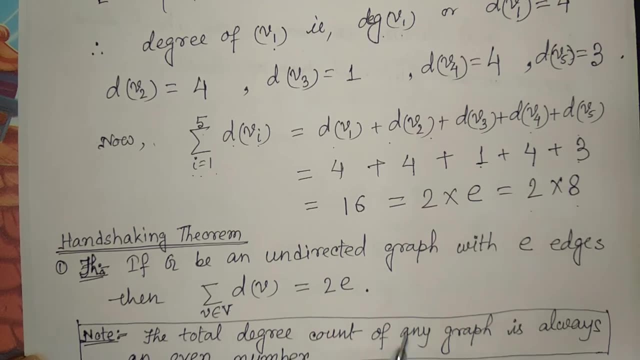 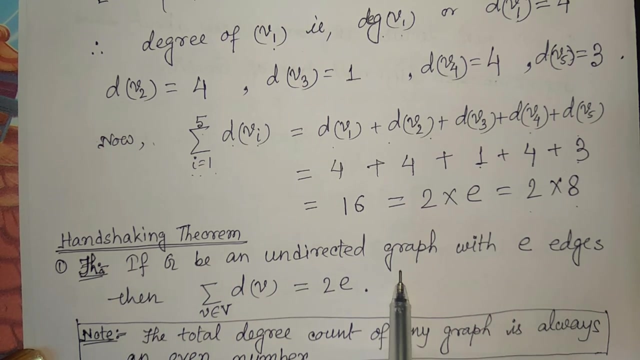 twice of the edges that we will find out Using this one. we have a great theorem in graph theory. The name of this theorem is the hand shaking theorem. The theorem statement is: if G be an undirected graph with E number of edges, then total degree. 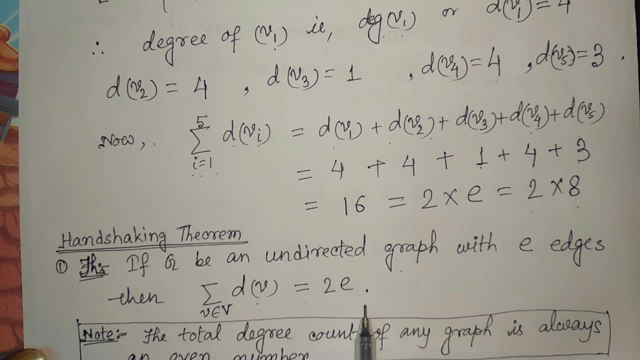 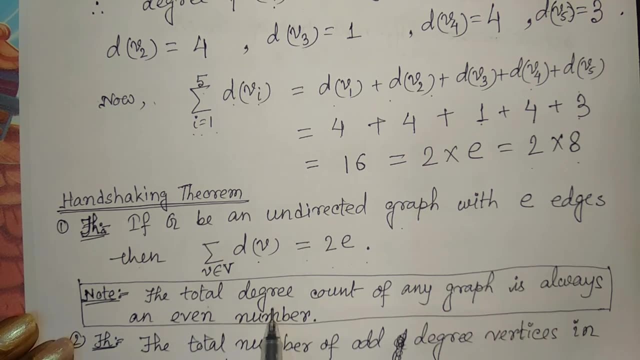 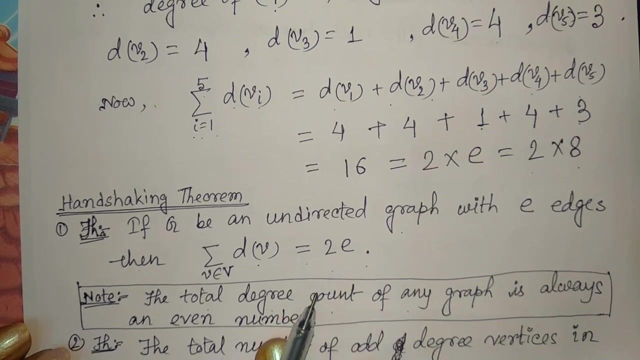 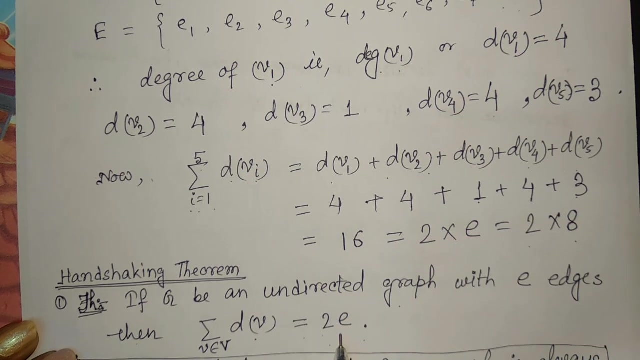 count of the graph is twice the number of edges. From here we can draw a conference that the total degree count of any graph is always an even number. And it is very true, because whenever we will count every odd degree, then it is always a multiple of 2.. Whatever be the number of edges, it is. 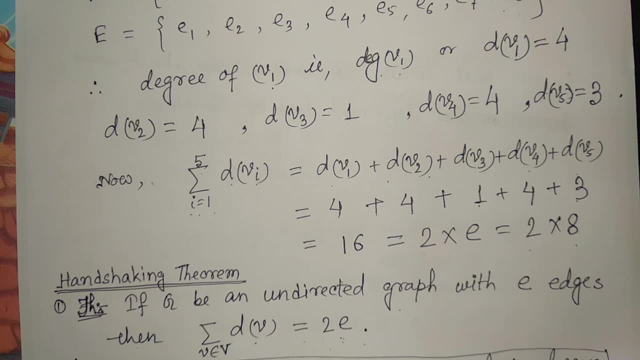 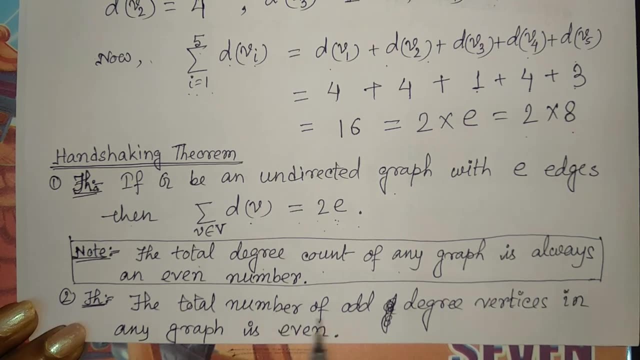 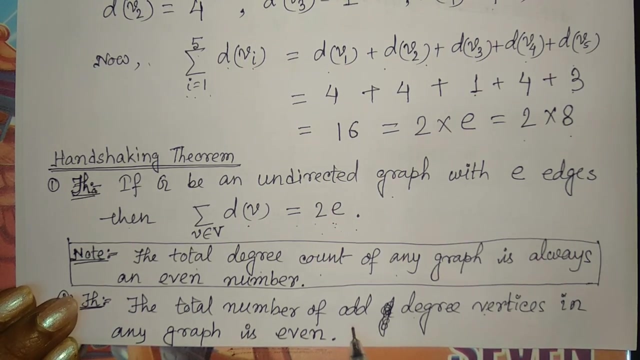 the multiple 2, so that always an even number. From here one more theorem we can draw, and the statement of this theorem is that the total number of odd degree vertices in any graph is even. So here we will find out one more term, ie the 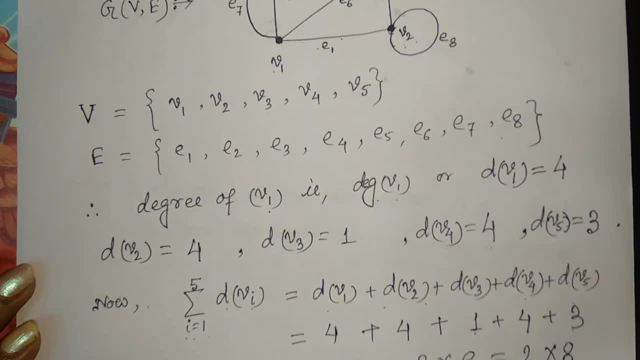 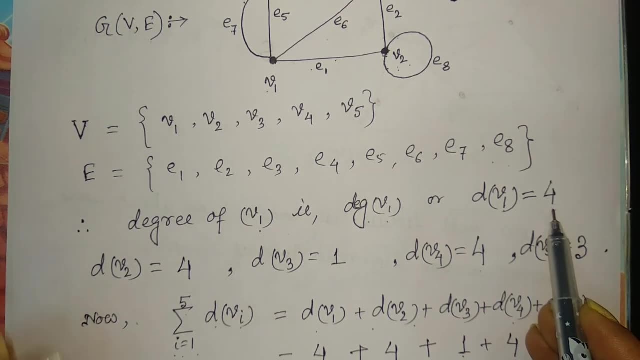 odd degree vertex. What so you mean by the odd rze degree? watch your brain look. in this given graph, the degree for vertex V1 is 4.. This is an even number, So that we can say: V1 is an even degree vertex For V2, the degree is 4.. So V2 is also an even degree. vertex V3, its degree. 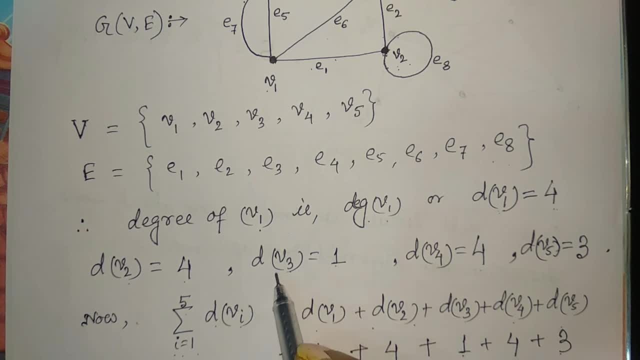 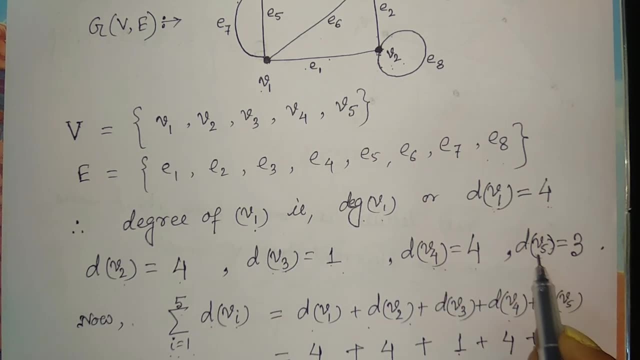 is 1, which is an odd number, So that we can say: V3 is the odd degree vertex For the vertex V4, the even number, So it is an even degree vertex, and V5, 3, it is an odd number. So 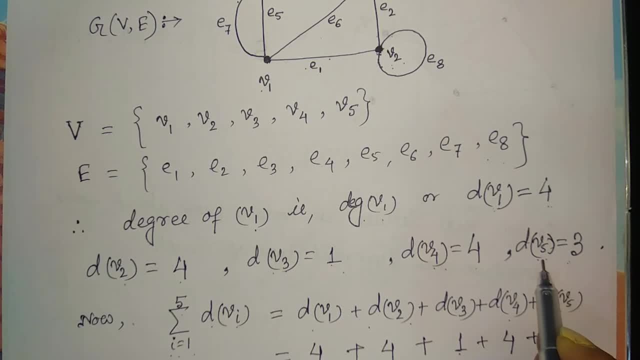 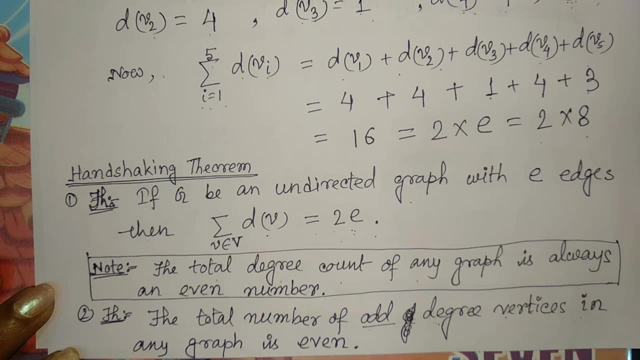 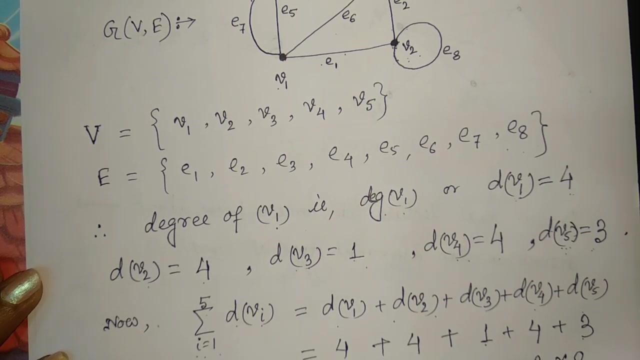 V5 also, we say it is an odd degree vertex. Now, according to the theorem, we have that the total number of odd degree vertices in any graph is even, And it is very obvious that we know that even even is even number. Odd plus odd is also even number. 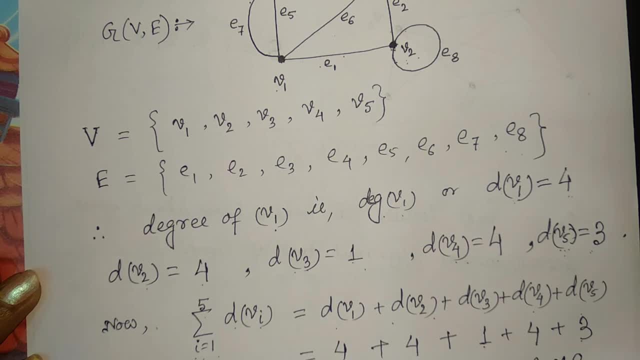 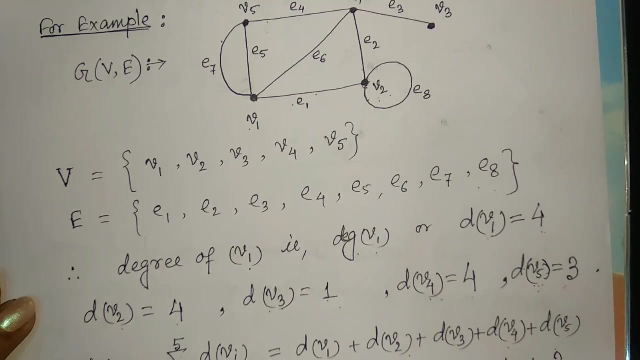 Odd plus even is odd number. Our total degree count is even. That's why if odd degree vertices are odd in number, then we will never get a even number as a summation. That's why if any odd degree vertex exist in the graph then it has to be even number. Now, the degree of a vertex. 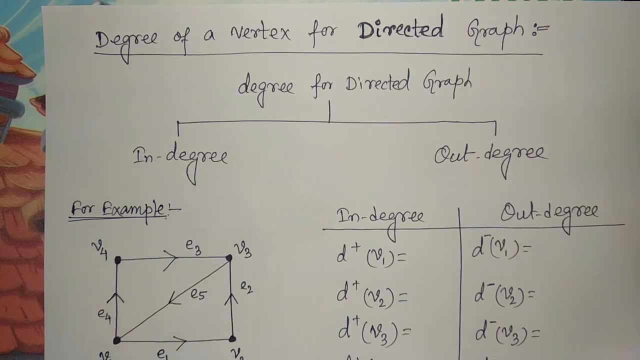 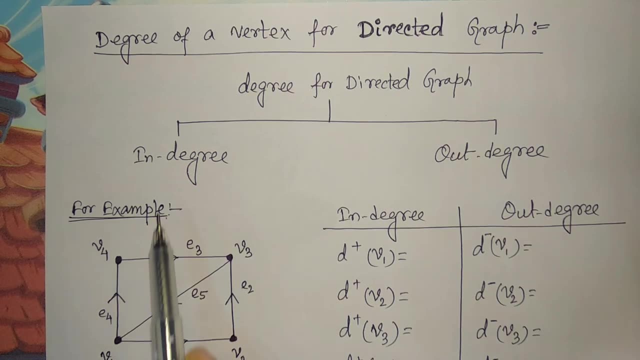 for directed graph. We know in our previous lecture what is the directed graph. So for directed graph, we will find out two type of degrees. One is called the in degree, another one is called the out degree. So what is this? in degree and out degree? 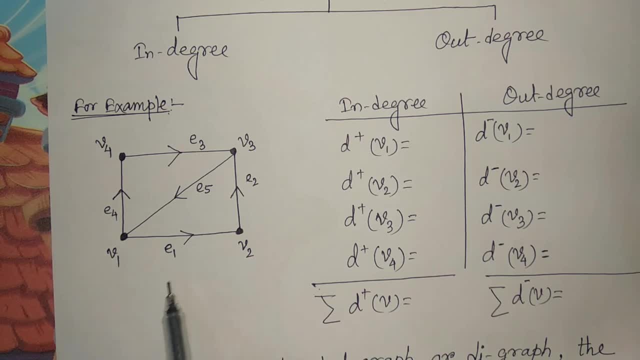 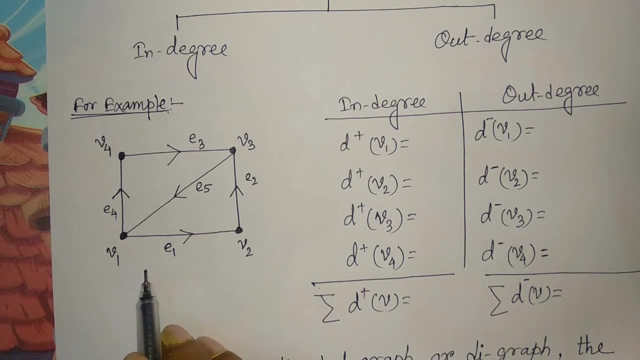 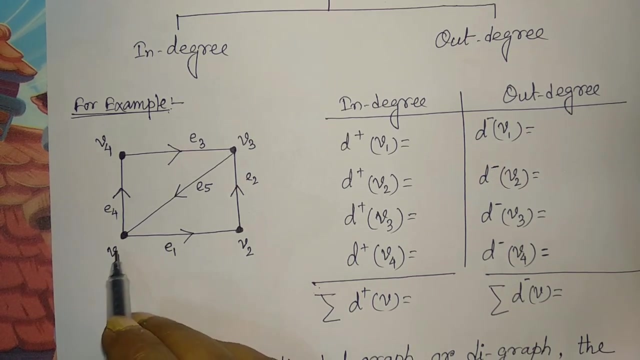 For example, suppose this one is our given picture- Here, total four vertices are there. So, corresponding to all these four vertices, we can calculate the degrees Here, the in degree and out degree, depending upon the direction of the edges, Here for V1, the even edge for 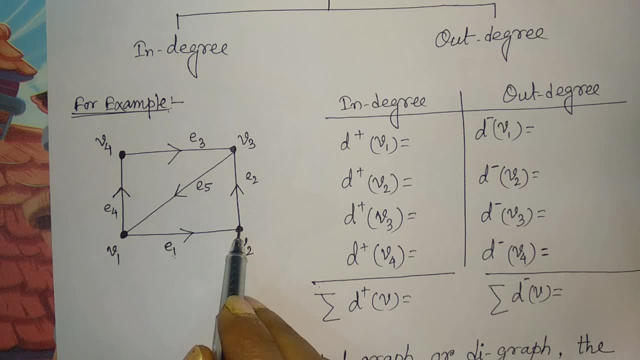 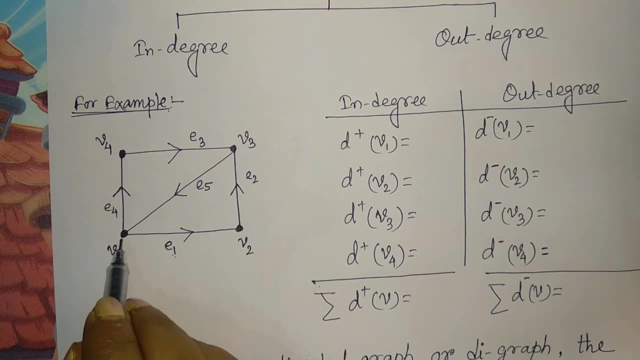 V1 is the starting vertex and V2 is the end vertex as it is a directed edge. For any directed edge we can calculate the in degree and out degree. So for V1, we can calculate the in degree and out degree. Now we can calculate V2 and V3 are the starting vertex, The vertex. 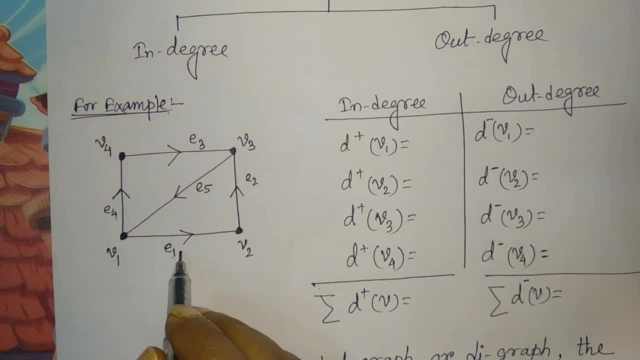 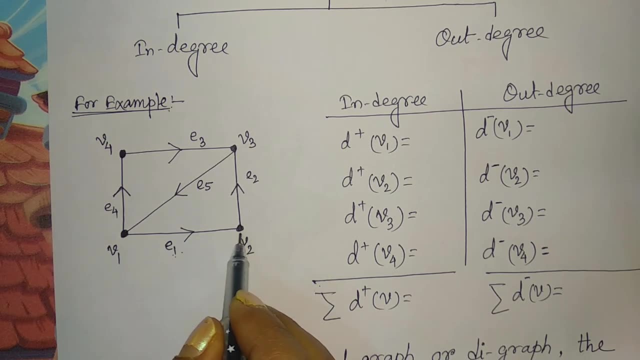 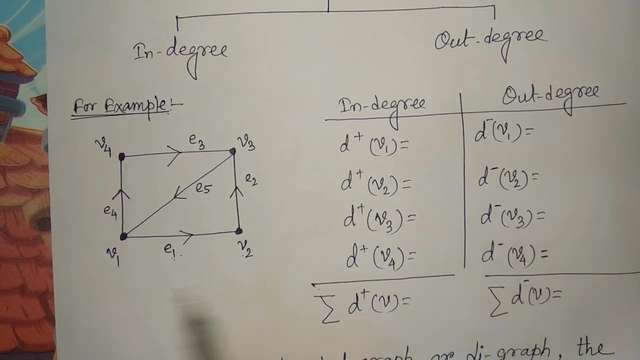 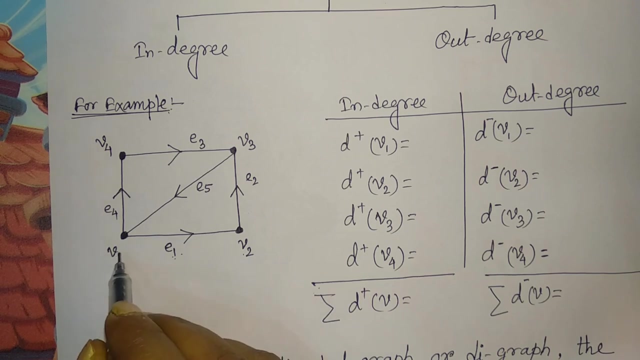 which have the starting vertex for any edge, that one will get the out degree corresponding to that edge and where it is the end vertex that one will get the in degree In easy manner. we can say that wherever the edge is entering into a vertex, that will gives the in degree. and if one edge is going out from a vertex then it will get the in degree. So, for example, the vertex which is out of the index then it will get the in degree. if i change the the edge into the beginning, If the edge is going out of the index, this will get the in. 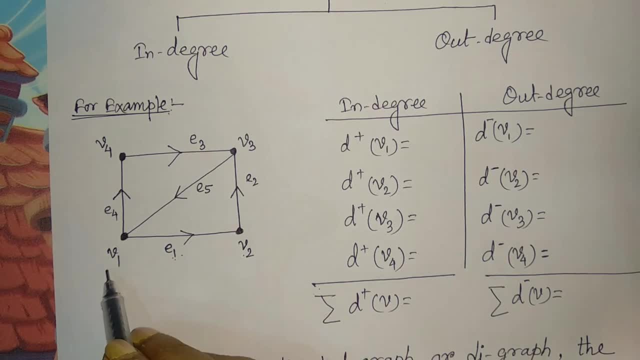 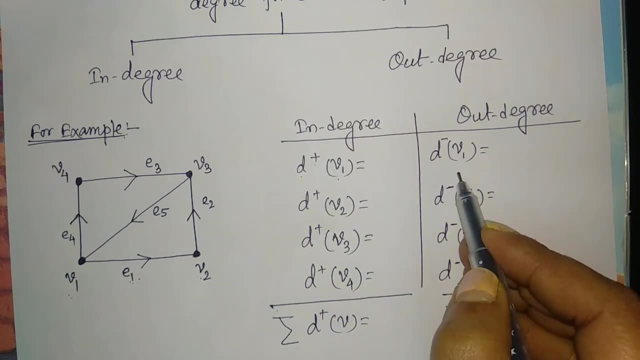 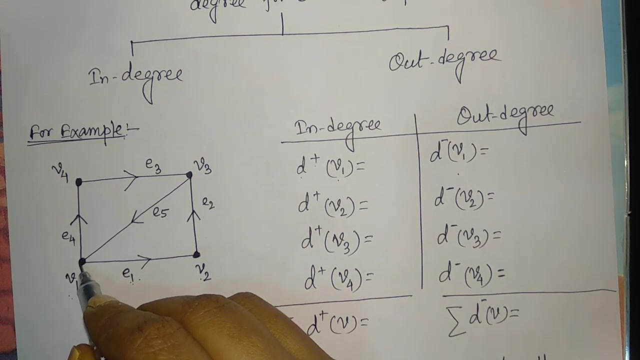 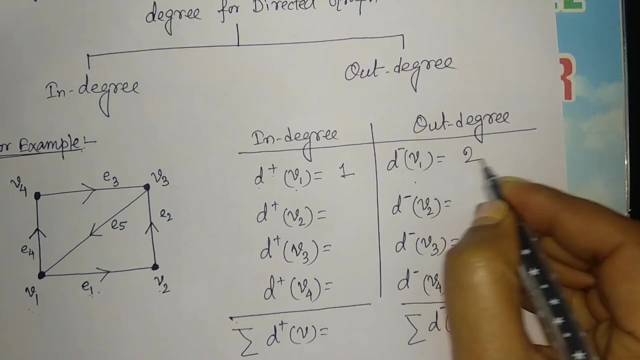 provides the out degree. So according to that concept for the vertex V1, we denote the in degree as D plus sign and out degree D minus sign. So for V1, the in degree, here only one edge is coming in to the edge V1. So in degree is 1 and out degree is 2.. Accordingly, for the vertex V1,, 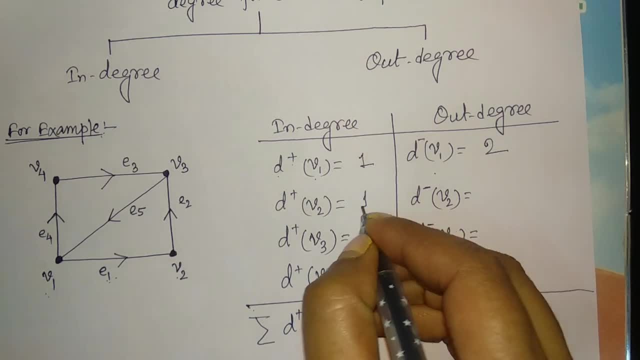 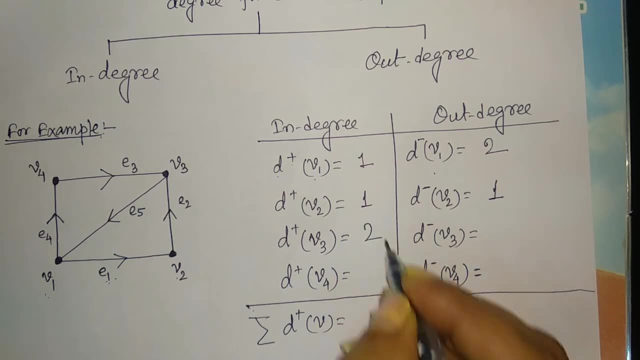 the in degree is 1 and the out degree is 1.. For the vertex V3, the in degree is 2 and the out degree is 1.. For the vertex V4, the in degree is 1 and the out degree is 1.. So this is the in degree. 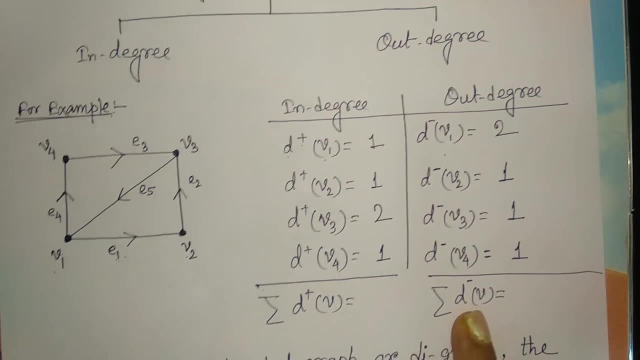 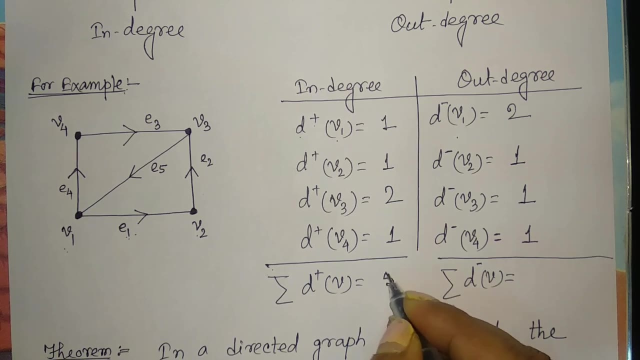 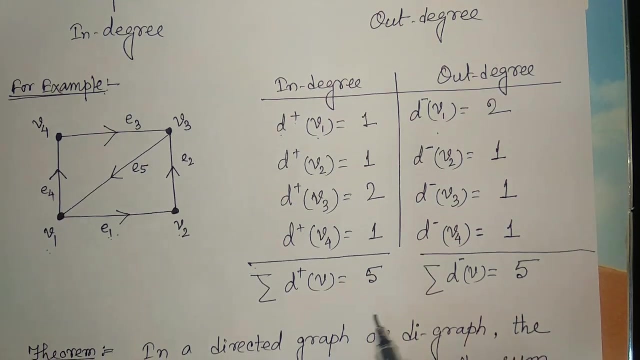 and out degree for the individual vertices. Now we can add all these in degrees. If we add all these in degrees, we can add all these in degrees. So this is the in degree and out degree for the in degrees. Then the total sum is 5 and total out degree sum is that is also 5.. So this 5 is the. 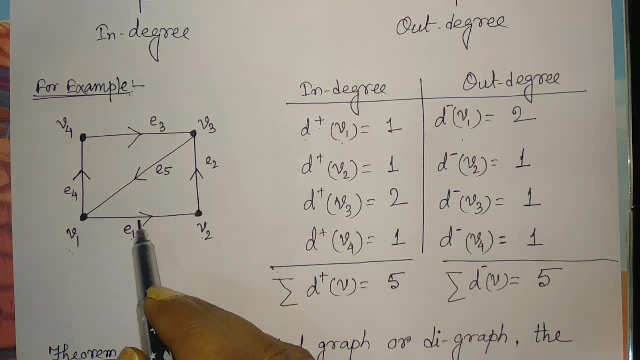 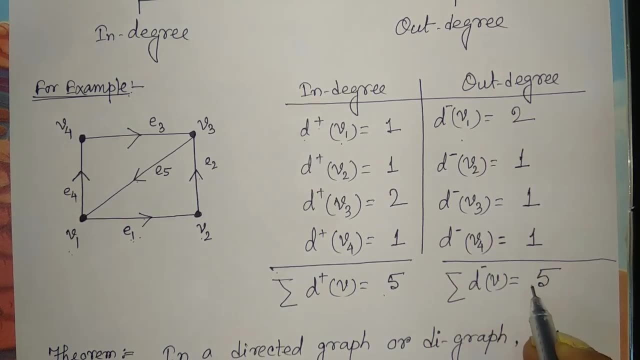 total number of edges. Look at the graph here. The total number of edges are 1,, 2,, 3,, 4 and 5.. So the total number of in degree and the out degree both are same and this count is exactly. 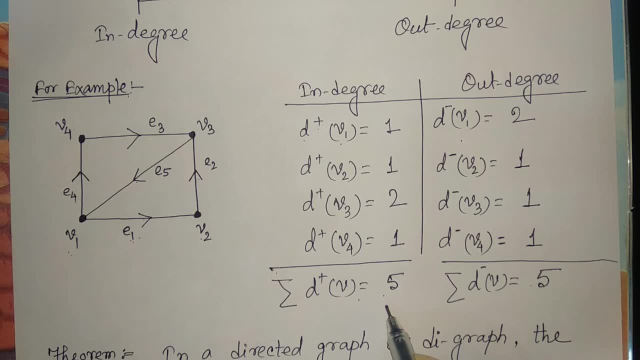 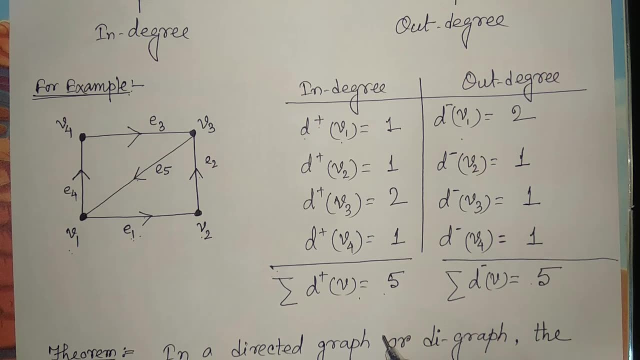 equal to the number of edges. It is very obvious, because 1,, 2,, 3,, 4 and 5 are the same. So because 1 edge contributes 2 degree to the graph and if it is directed graph then 1 edge. 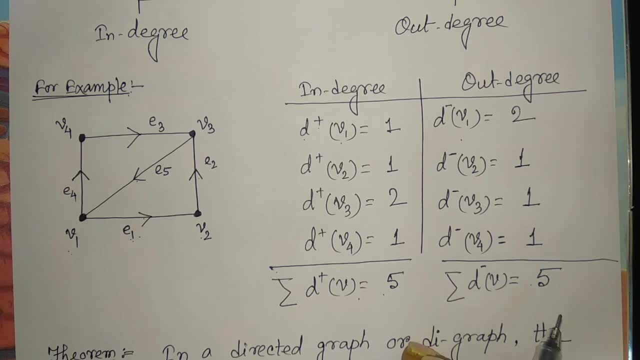 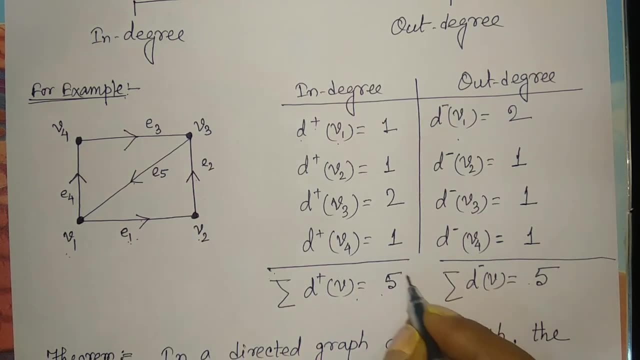 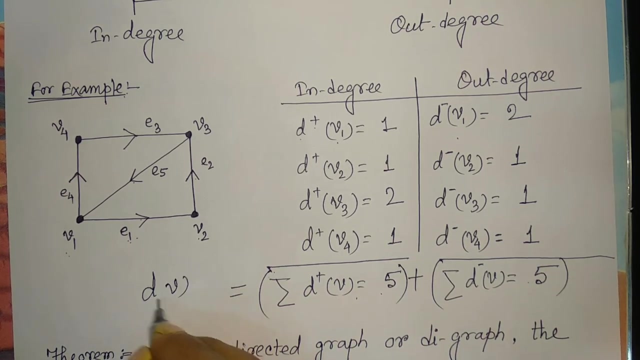 contributes 1 in degree and 1 out degree in the graph. Hence, always the number of in degree and the number of out degrees are same, and if we add this number of in degrees and out degrees then we will find out the total degree count for the graph According to this one. 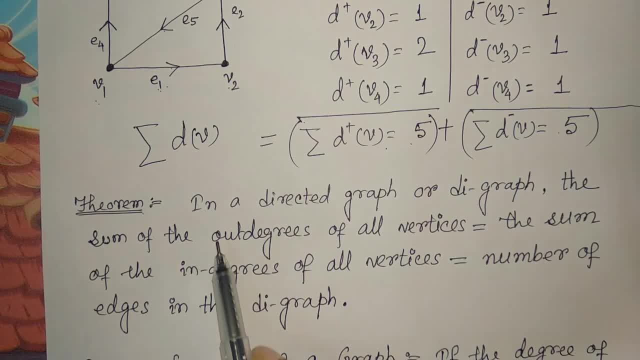 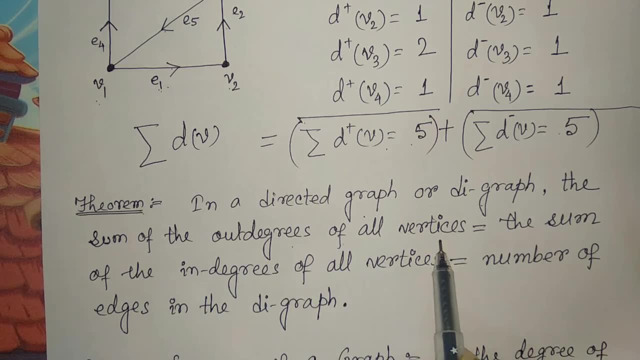 our theorem for the in degree and out degree. the theorem is in a directed graph or digraph. the sum of the out degrees of all vertices equals to the sum of the in degrees of all vertices, equals to the number of edges in the digraph. Now we have another thing, that is: 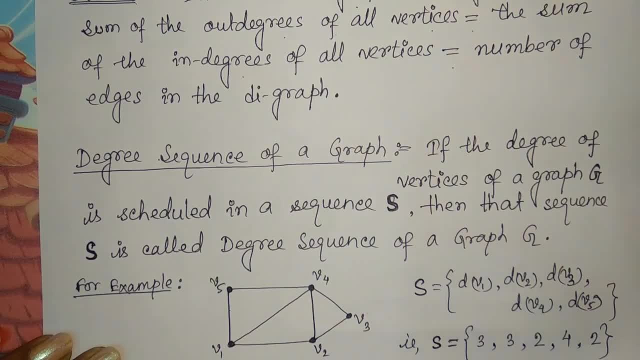 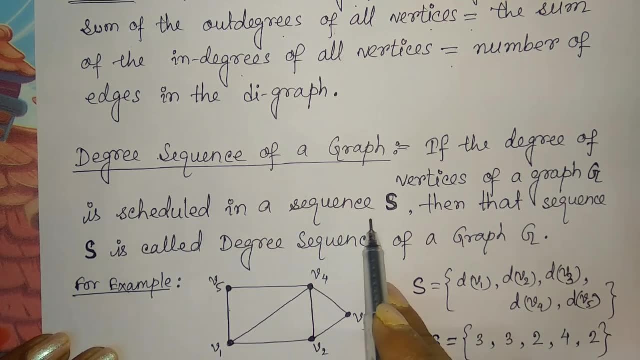 called the degree sequence of a graph. So what do you mean by the degree sequence? If the degree sequence of a graph is equal to the number of edges in the digraph, then the degree of vertices of a graph G is scheduled in a sequence S, then that sequence S is called. 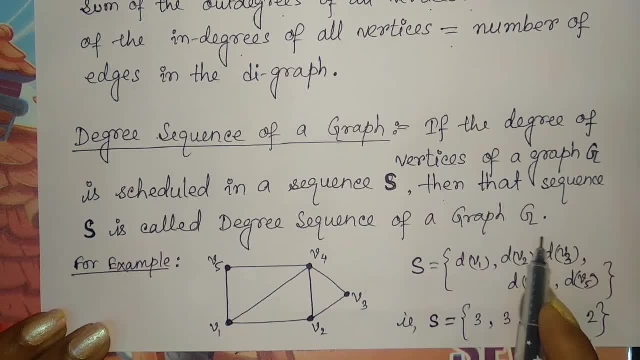 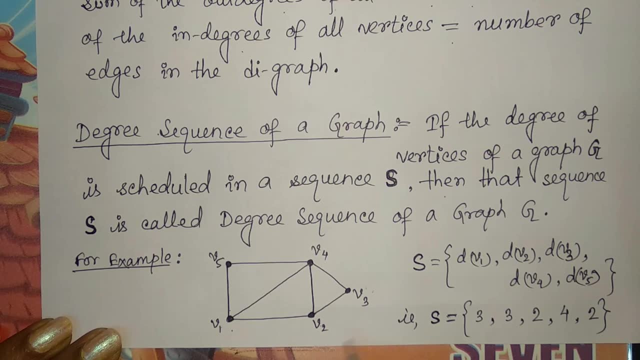 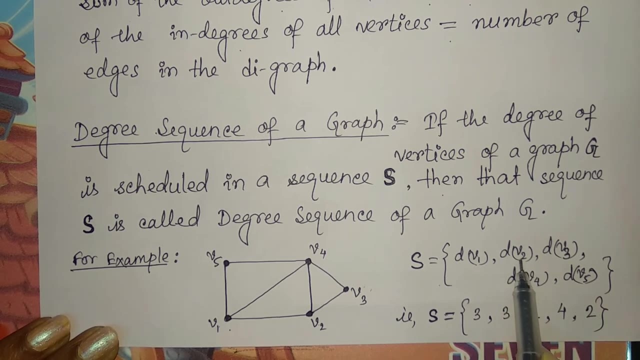 degree sequence of the graph G, For example. let this one is the graph. Here total 5 vertices are given. So for these 5 vertices we can write a sequence format using their degrees. So S is equal to dv1, dv2, dv3, dv4 and dv5.. 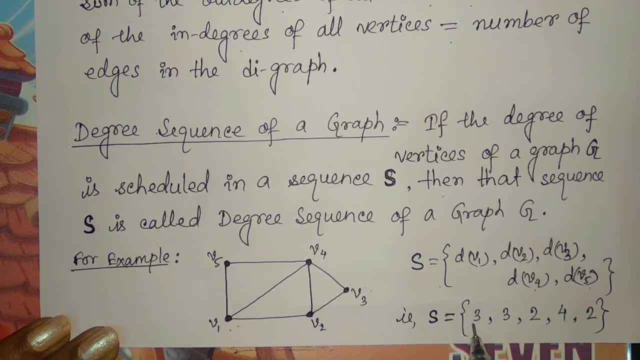 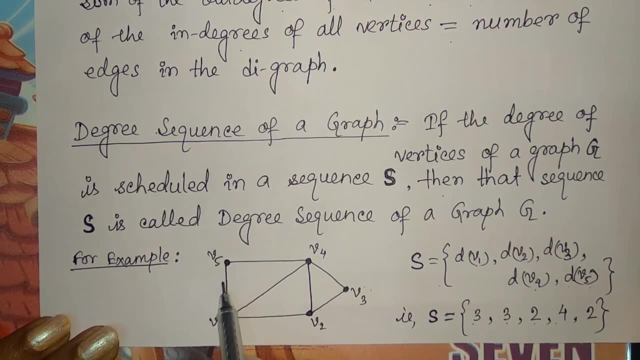 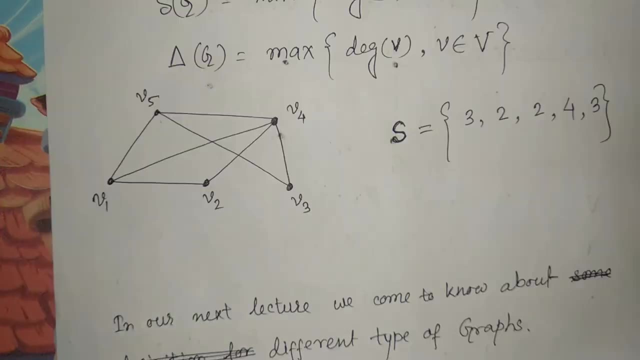 The degree of v1 is 3.. That's why it is 3.. Degree of v2 is also 3.. Degree of v3 is 2.. Degree of v4 is 4 and degree of v5 is 2.. So this is called the degree sequence of the graph. Now one more thing. 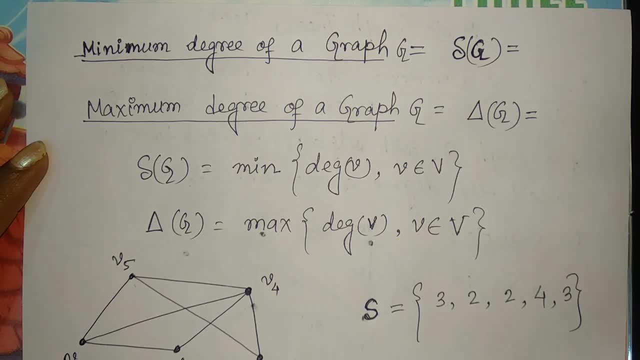 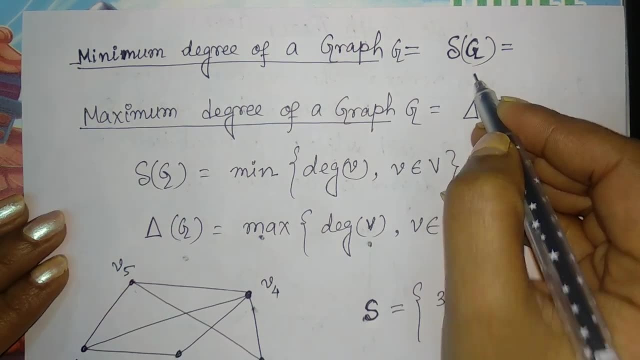 is there. That is the minimum degree of a graph. G That is denoted by delta G. So what do you mean by the minimum degree? So minimum degree of the graph, not the vertices. So minimum degree of graph means whatever the 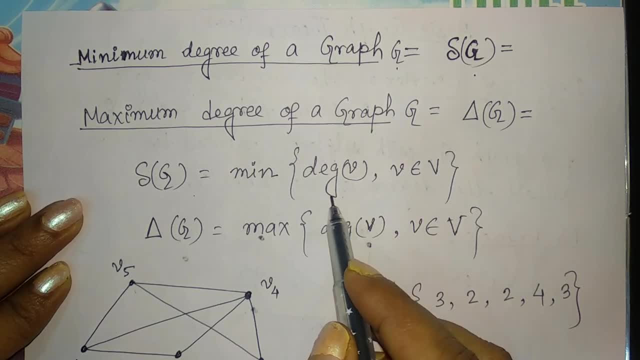 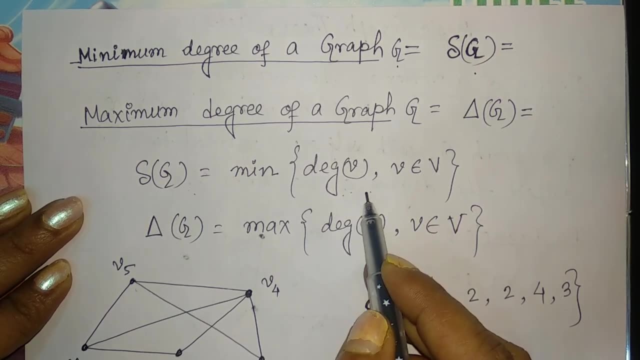 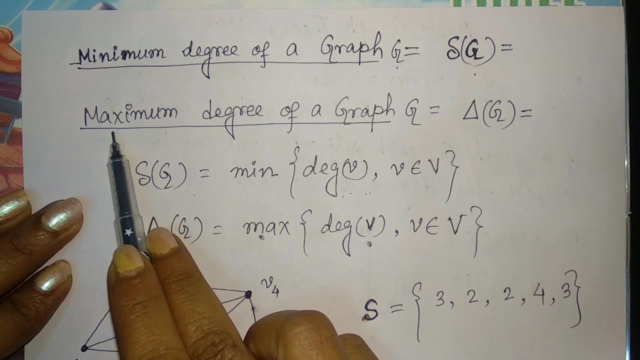 degrees you have calculated for the entire graph, for each individual vertices, all those degrees among which vertex have the minimum degree, That one. that value is the delta G value. Here one thing is more: maximum degree of a graph G, which is denoted by big delta G.